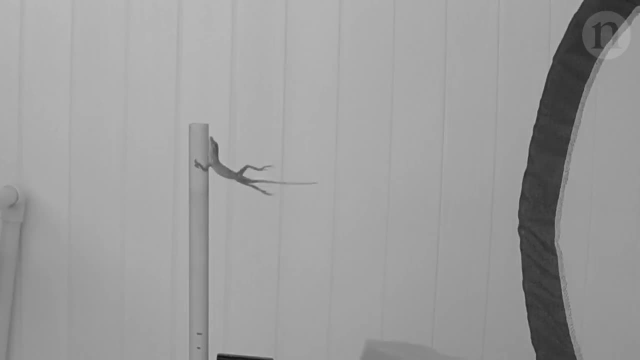 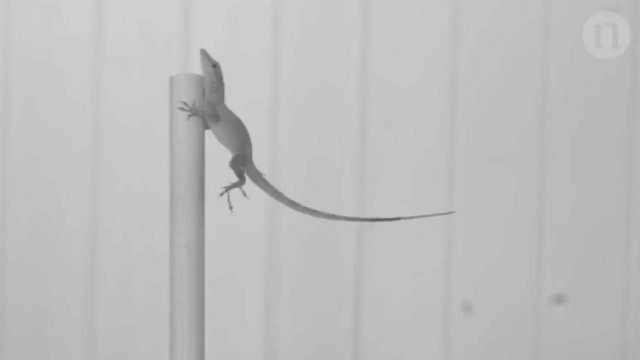 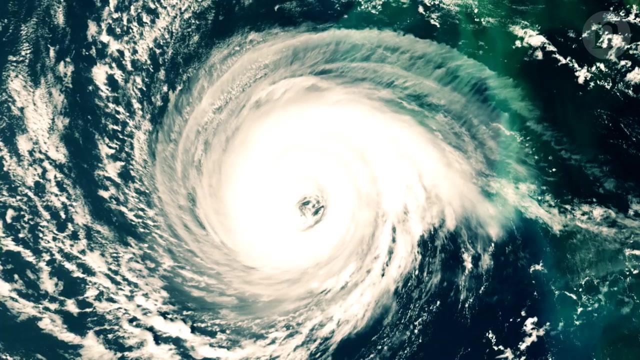 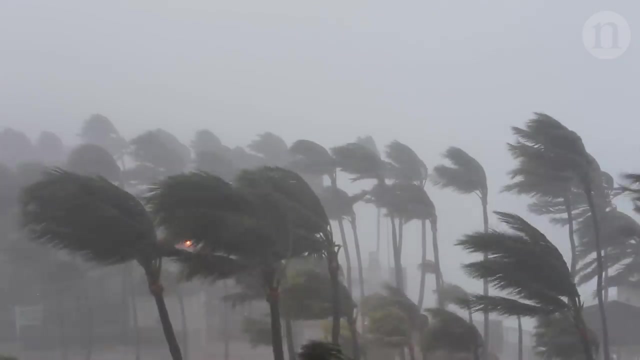 These lizards are leaping- for science, Well, not so much leaping as falling, But their tumbles are helping scientists answer a question: Could hurricanes drive natural selection? Hurricanes are destructive, perhaps too destructive to influence evolution, with species survival being more random than influenced by specific traits. And while some scientists suspect, 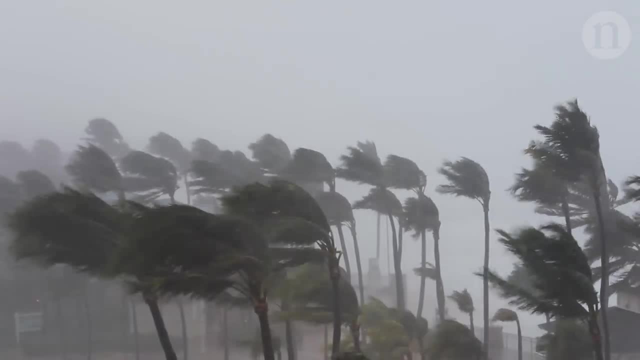 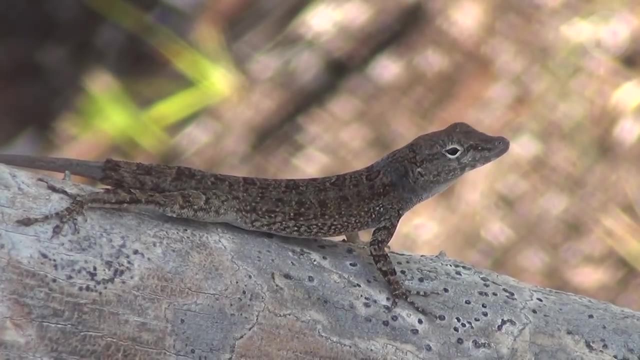 that hurricanes could drive natural selection. this has never been documented, That is until a group of researchers happened to be measuring anole lizards in the Caribbean. They surveyed lizards on two small islands in Turks and Caicos just days before Hurricanes Irma and 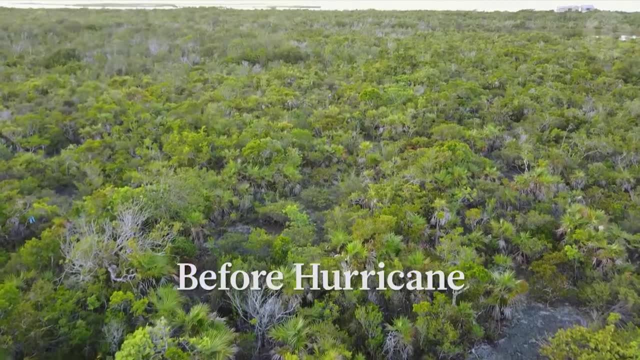 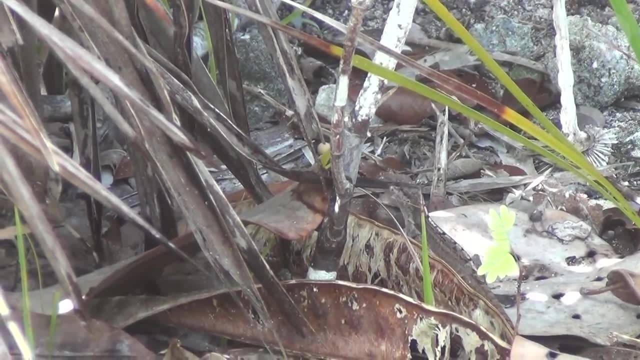 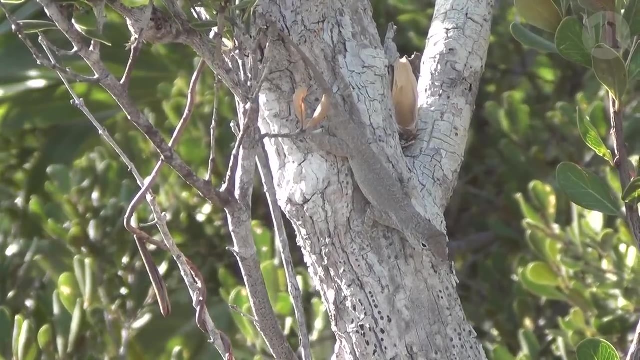 Maria struck. Winds reached speeds of more than 200 kilometers per hour, felling trees and flattening vegetation. But after the devastation, the scientists had a rare opportunity to see how the hurricanes affected the lizard populations. They went back and measured the lizards left on the 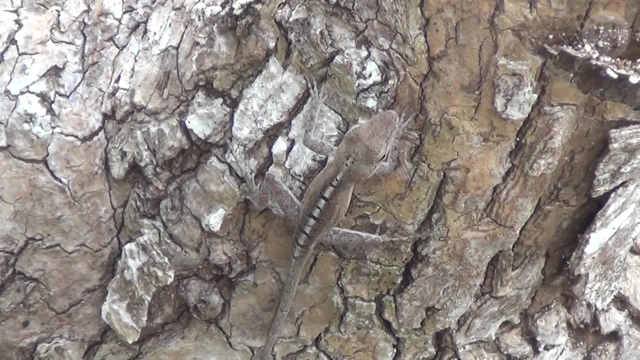 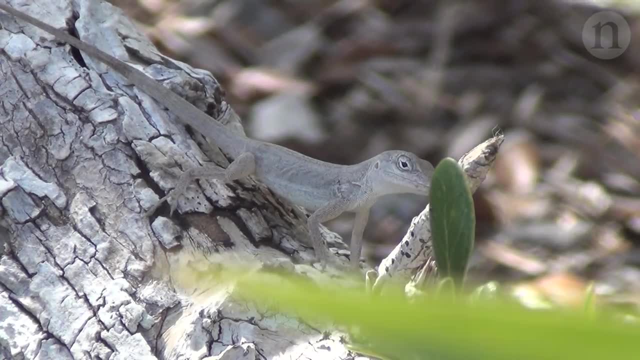 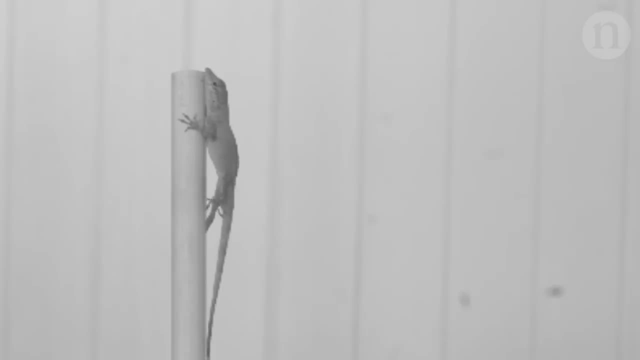 islands. On average, those that survived had larger toe pads and shorter femurs. The males also had smaller bodies. Researchers suspect that these small differences might help the animals cope with the changes in their lives. But how Well that brings us back to lizards falling into nets. This simple test done. 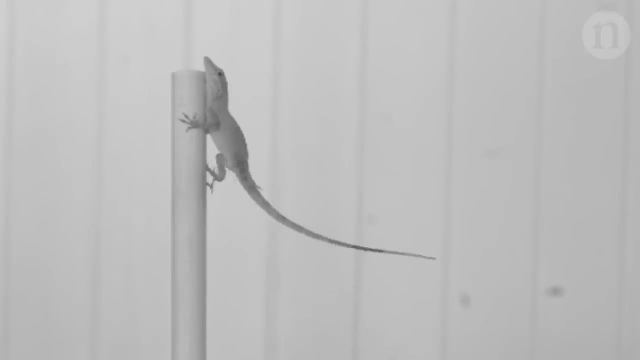 with a leaf blower demonstrates how they respond to high wind. To stay on the branch, the lizards tuck their forelegs under their body and out of the wind, But their hind legs stick out, catching the wind until they ultimately lose their grip. The scientists say that shorter 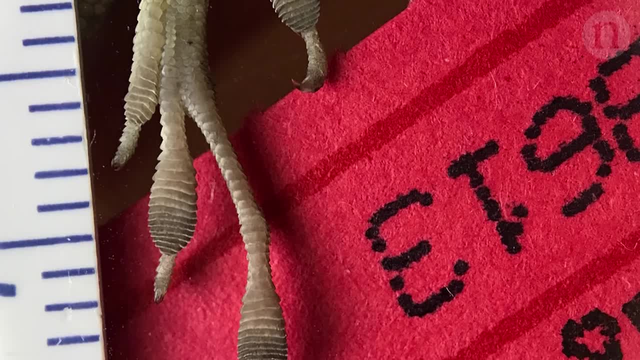 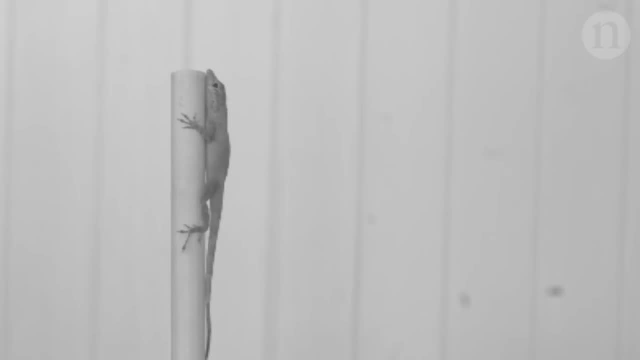 femurs and smaller bodies are more likely to get caught in the wind than in the wind. Additionally, the lizards' toe pads are covered in tiny ridges. Larger pads means more ridges and so better grip. Right now this is mostly speculation, but it could explain the differences. 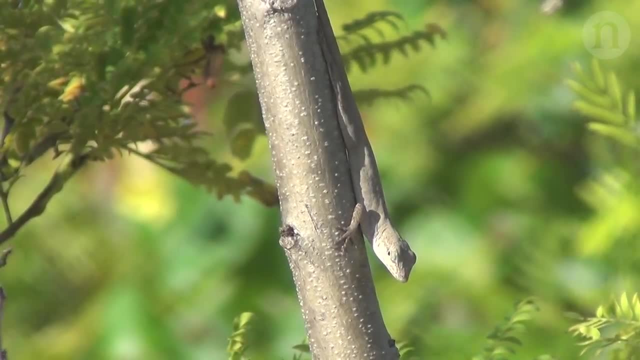 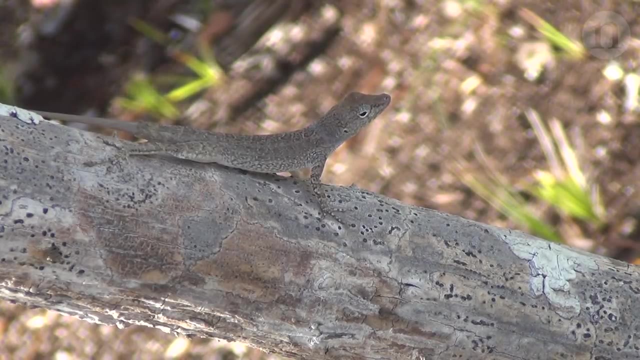